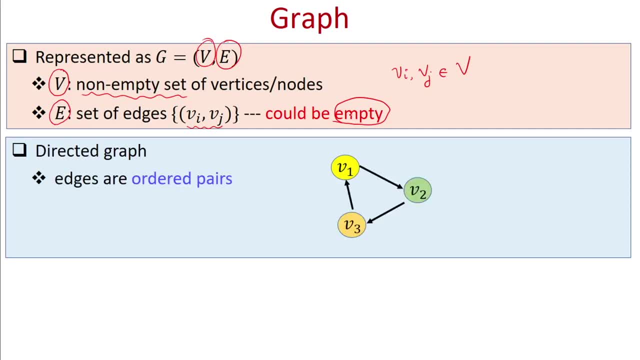 When I say directed graphs, then pictorially you can imagine that in directed graph the edges have directions associated with it. That means we have the notion of the starting point of an edge and the ending point of an edge And in terms of set theoretic notations, 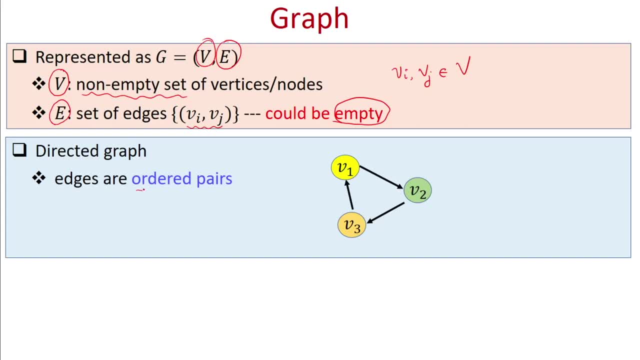 we can say that a direct edge is a set of edges And, in terms of set theoretic notations, we can say that a directed graph is a graph where the edges are ordered pairs. And as soon as I say that edges are ordered pairs, 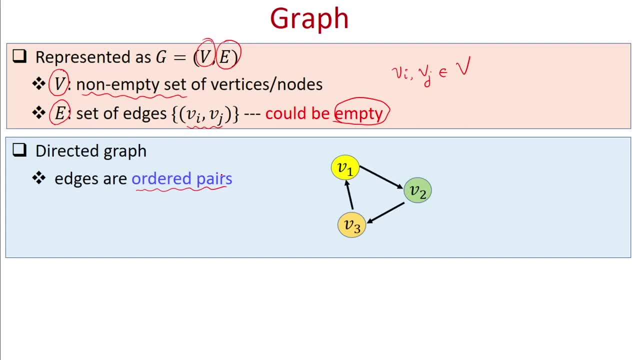 that means it matters whether the starting end point is VI or the starting end point is VJ, If you're talking about an edge VI, comma VJ, right. So, for instance, if I consider this directed graph, and the edges that we have here are the ordered pairs: 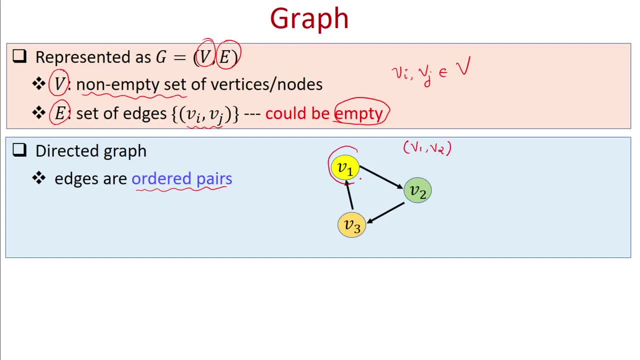 V1 comma V2, because the starting point of this edge is V1 and the end point is V2.. We have, but that does not mean that in the graph we also have the edge from V2 to V1, because that edge is not there explicitly in this directed graph right. 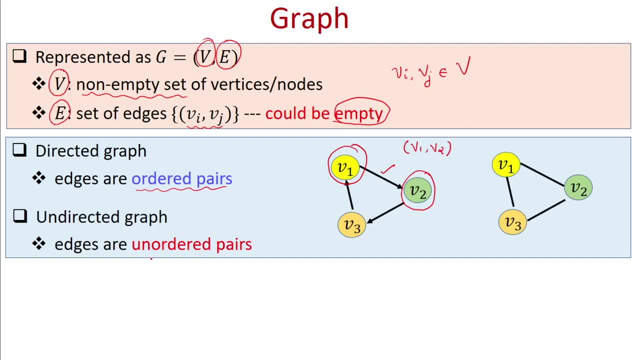 Whereas if we consider undirected graphs, then the edges have no direction associated with them, which is equivalent to saying that the edges are unordered pairs. That means, when I consider this edge from the vertex V1 to vertex V2, it can be also considered as an edge from V2 to V1.. 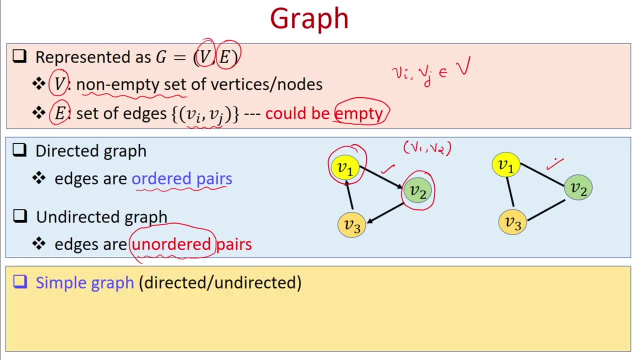 In that sense, the edges are here bidirectional. OK, so let us now define what we call as a simple graph, And this definition is applicable both for the directed graph as well as undirected graph. So a simple graph is a graph which has no self loops. 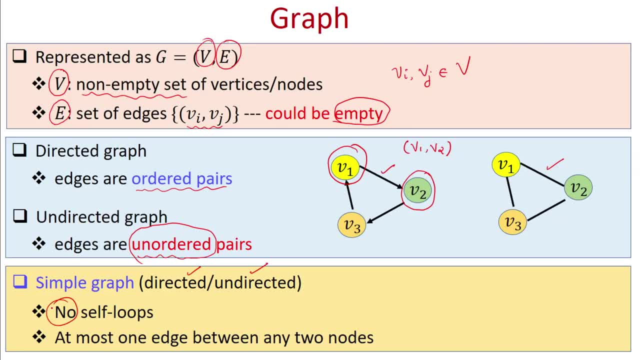 OK, and there can be at most one edge. between any two edges, There can be two nodes, OK. so if I consider this undirected graph, then this is not a simple graph, because between the nodes V1 and V3, you have two edges: this edge as well as this edge. 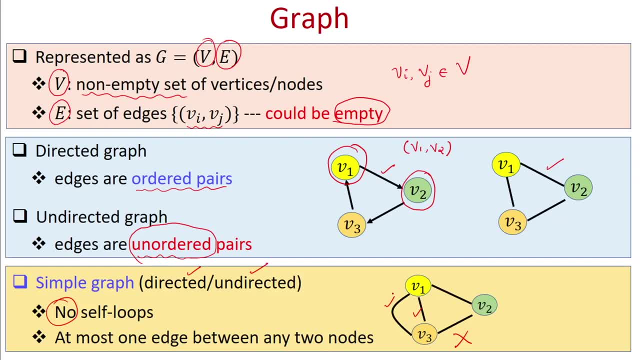 which is not allowed as per the definition of an undirected simple graph. But if I consider this directed graph, then this is a simple directed graph because, even though you have two edges involving the nodes V1 and V3, this is one of the edges and this is another edge. 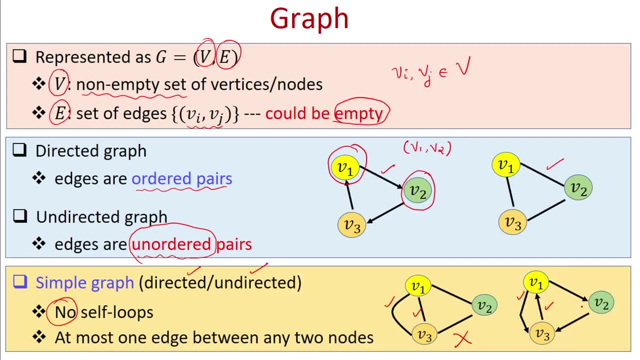 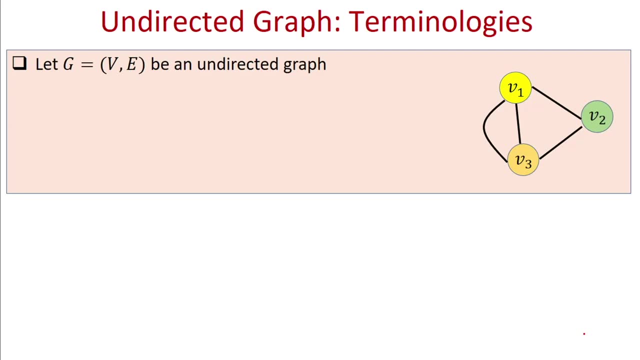 They are different directed edges because the ordered pair V1, V3 will be different from the ordered pair V3, V1.. So this is an example of a directed simple graph. OK, so now let's introduce some terminologies related to undirected graphs. 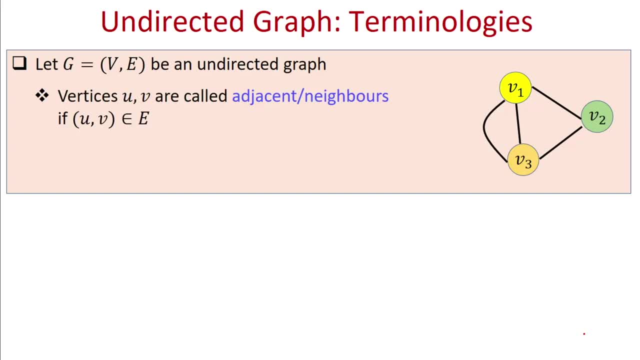 So if you are given an undirected graph, then a pair of vertices, U- V, are called adjacent or neighbors of each other. if the edge U- V belongs to my edge set, OK, that means if U and V are the end points of an edge, then in an undirected graph 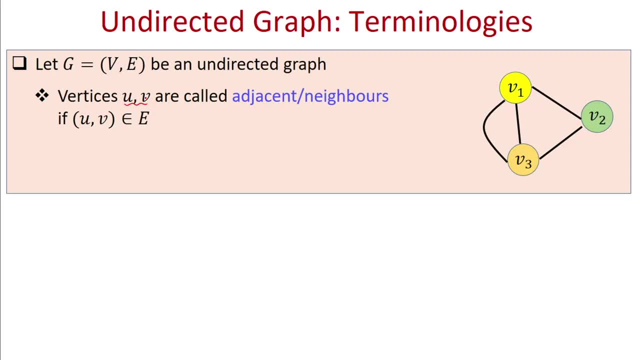 then we call the vertices U and V to be adjacent or neighbors. OK, here V could be U, that's allowed. That means if I have a self-loop, then the vertex V will be called adjacent to itself. right. Then if we are given an edge small e. 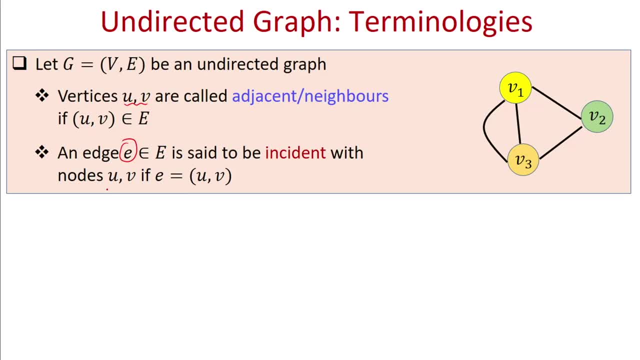 then we will say that it is incident with the nodes U, V if U and V are the end points of the edge. So, for instance, if I consider this edge small e, then V1 and V2 are incident with respect to this edge. 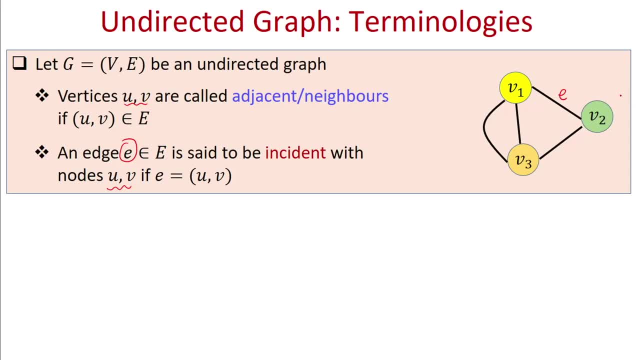 because they are the end points of this edge, E and so on. Now let us define next what we call as the degree of a vertex, small v. So again, I'm giving the definition with respect to undirected graph, but the definition can be extended or generalized for directed graphs as well. 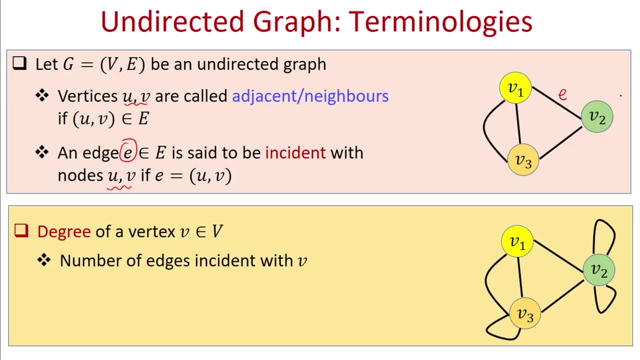 OK, so what is the degree of a vertex? The degree of a vertex is the number of edges incident with V or, in simpler language, the number of edges which have small v as one of its end points. OK, and the definition has a special case. 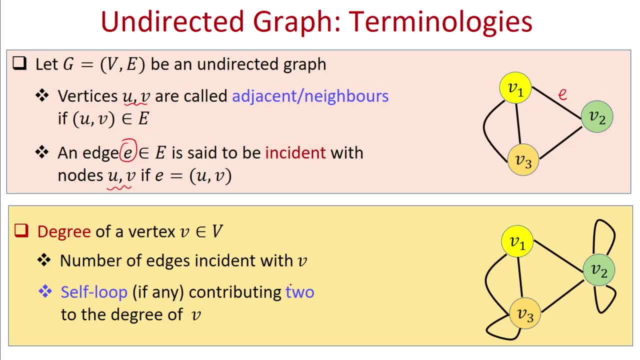 If we have a self-loop incident with the vertex small v, If there is a self-loop incident with the vertex small v, then that self-loop is counted as contributing 2 to the degree of the vertex small v. OK, so, for instance, if I take this undirected graph and the degree of the 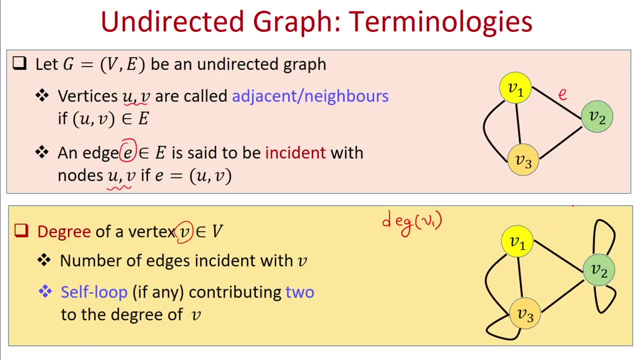 vertex V1, let us find out what's the degree. So how many edges are there? incident with the vertex V1?? So this is one of the edges, This is another edge to the 2 edge, And now we have this edge again. incident with V1. 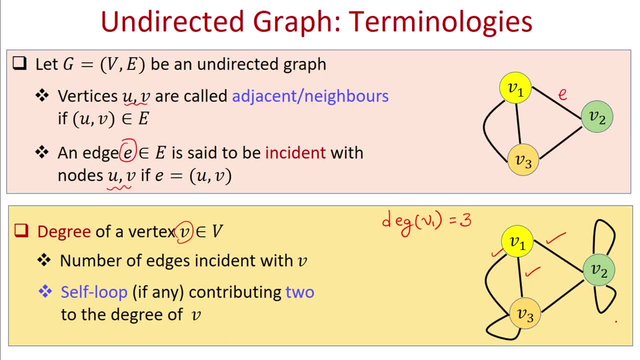 So total 3.. Whereas, if I consider the degree of the vertex V3,, then we have this edge, this edge, this edge, and we have a self-loop. The self-loop will be counted twice while counting the degree of the vertex V3.. 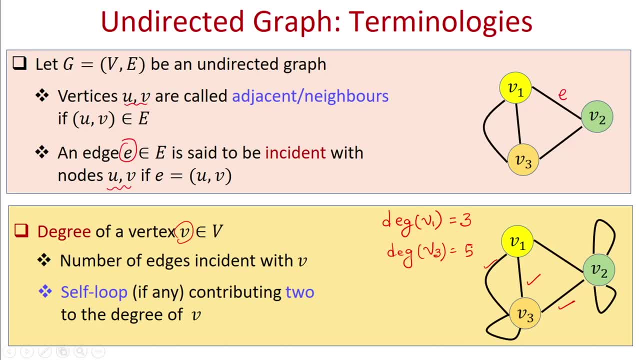 So, total, the degree of the vertex V3 will be 5, and so on. OK, so this degree of a vertex, the definition is with respect to the undirected graph. The undirected graph need not be simple. In fact, in this particular example, between the vertex V3 and V1, we have two edges. 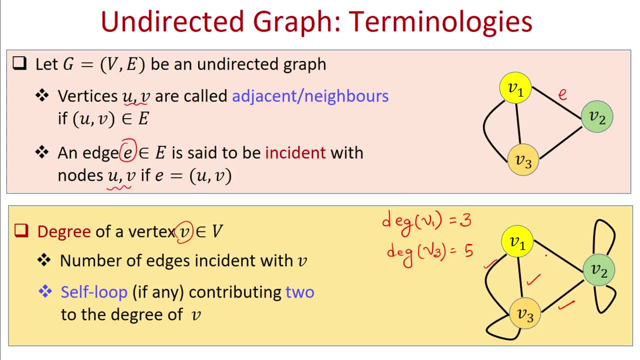 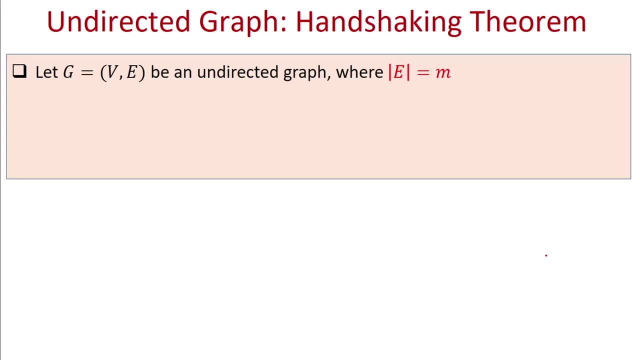 and both of them are counted. While counting the finding the degree of the vertex V3.. Next, we state a very fundamental fact about an undirected graph. This is also called as the hand checking theorem. So if you are given an undirected graph, it may be simple. 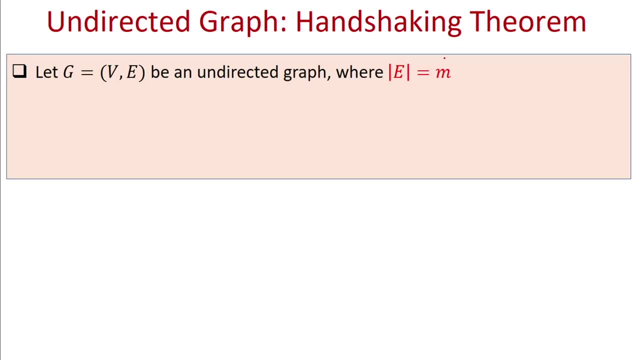 It may not be simple. It's just an undirected graph. and say the graph has M number of edges, Then what the theorem basically says is that if you sum the degrees of all the vertices in the graph, then it will be twice the number of edges always. 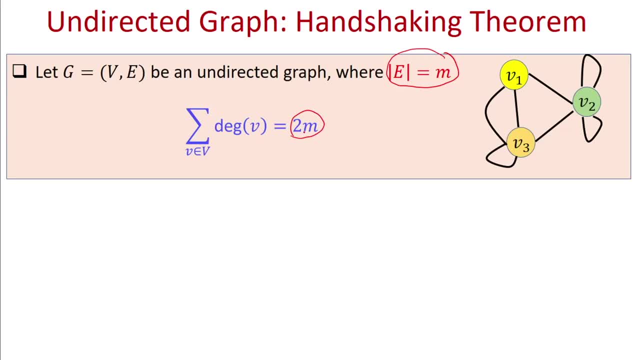 OK, so you can verify this. with respect to this example graph, You take the. so you take the summation of the degree of the vertex V1, the degree of the vertex V2 and the degree of the vertex V3. It will be equal to twice the number of edges in the graph. 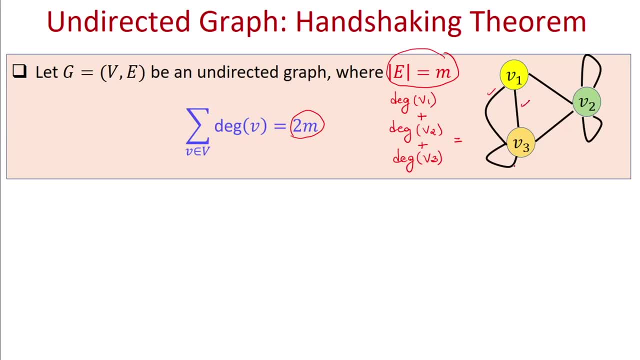 So what's on? So you have 1,, 2,, 3,, 4,, 5,, 6 and 7 edge. So 2 times 7 is 14.. And you can verify that the degree of V1 is 3.. 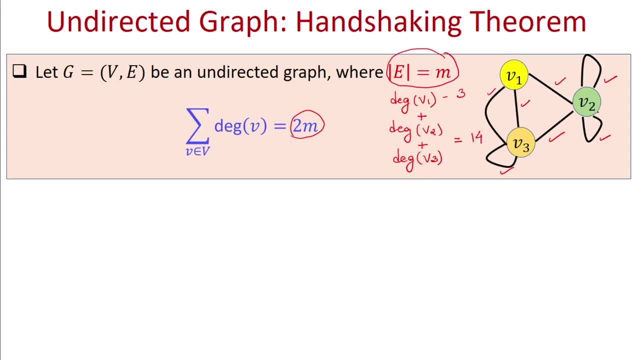 And degree of V2 is 2,, 4,, 5,, 6, degree of V2 is 6 and degree of V3 is 1,, 2,, 3 and 5.. OK, so let us prove this. 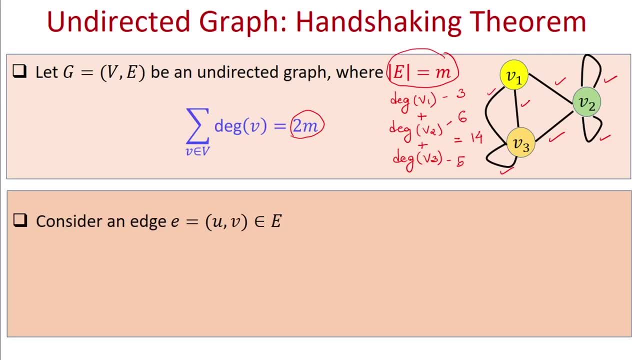 The statement is true for any undirected graph. So consider any arbitrary edge in your undirected graph: U, V. It may be a self loop, That means V could be same as U, or it may not be a self loop, And let us try to find out that. what will be the overall contribution of this? 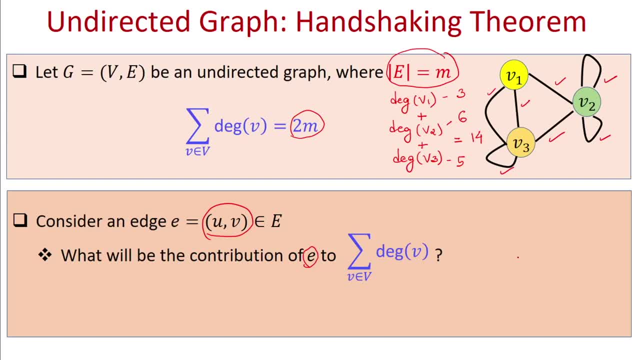 edge when we are summing up the degrees of all the vertices in the graph. So the claim is that the contribution of this edge will be 2 to the overall summation of degrees of all the vertices, because this edge will be contributing 1. 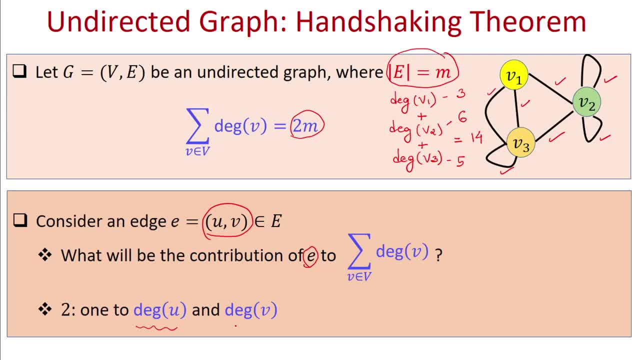 when we will be taking the degree of the vertex U and it will be again contributing 1 when we are taking the degree of vertex V. And if U is same as V then, as per the definition of the degree, the self loop will be counted twice, right, because U will be same as V. 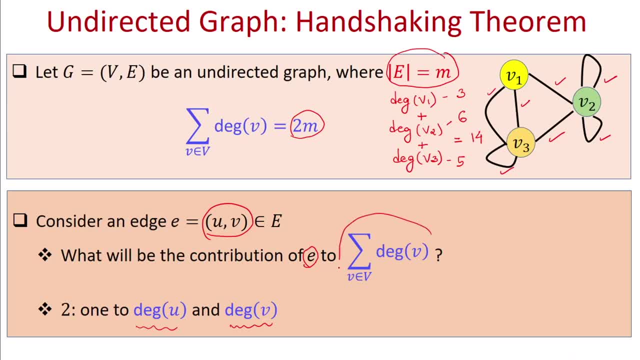 So that's why, in the expression, when we are summing up the degrees of all the vertices in the graph, the contribution of the edge U V will be 2.. And hence it's easy to see that the summation of the degrees of all 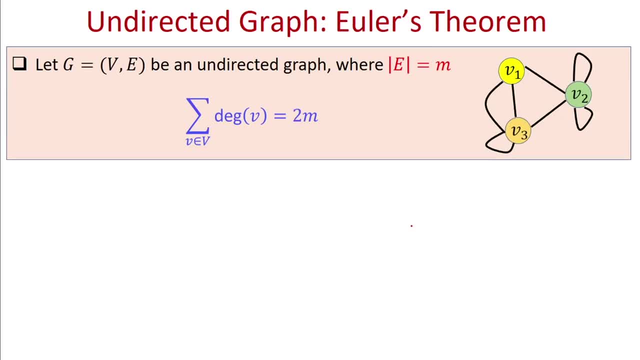 the vertices will be twice the number of edges in the graph. OK, so based on this fundamental fact, we can derive another conclusion about any undirected graph, and this conclusion is often called as the Euler's theorem. So what it says is the following: 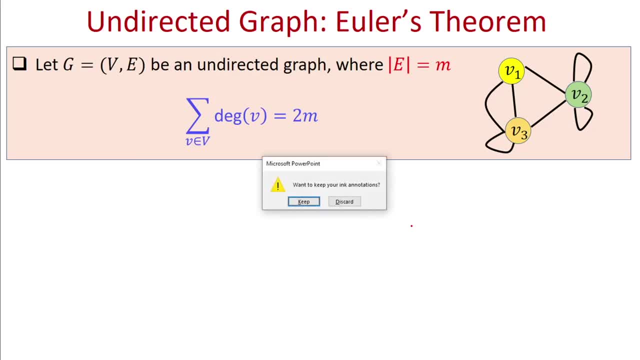 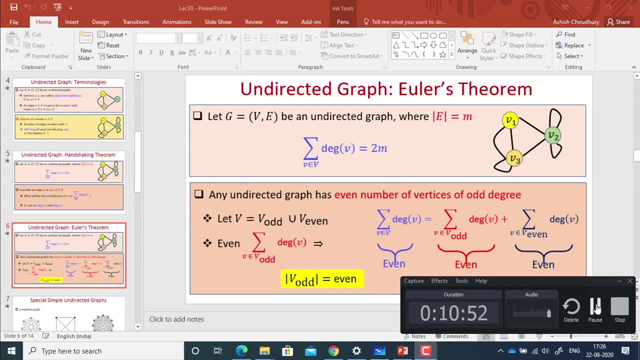 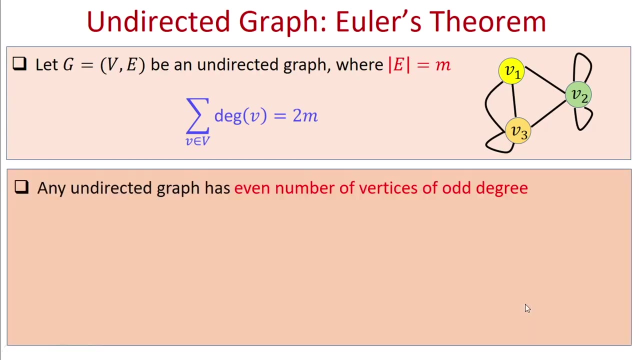 If you have. So what this theorem basically says? it says that you take any undirected graph, then the number of vertices of odd degree will be always even. That means you will either have zero number of vertices of odd degrees, or two vertices of odd degrees, or four vertices of odd degree, or so on. 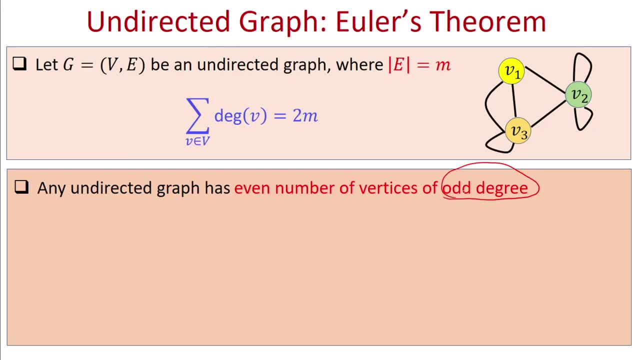 That means it won't be the case that the number of vertices of odd degree is odd, And for that, for deriving this conclusion, we will use the previous fact, namely the summation of the degrees of all the vertices in the graph is twice the number of edges. 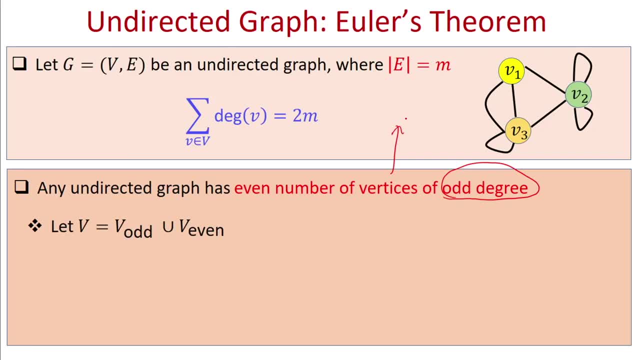 And the proof is very simple. So let V be the set of vertices In your undirected graph. the set V can be divided into two disjoint sets: The set V-odd, which is the set of all vertices which have odd degrees, and the set V-even, which is the set of all vertices which have even degree. 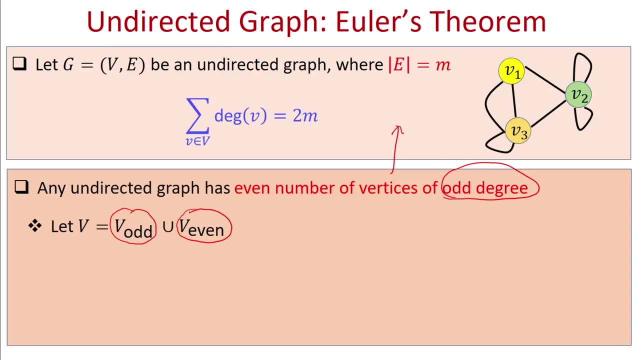 And it's easy to see that the intersection of these two sets will be empty, because you can't have a vertex in a graph which has both odd degree as well as even degree. So the vertex will have either odd degree or even degree, And hence it will belong either to the set V-odd or to the set V-even. 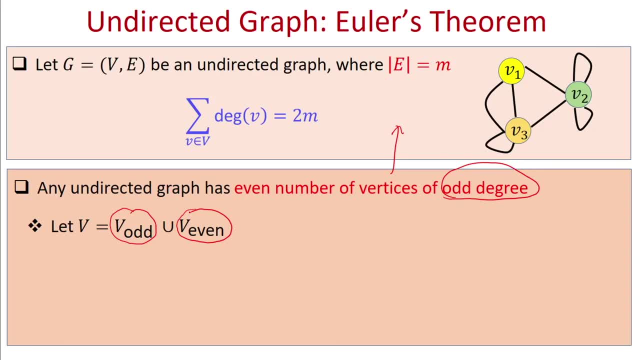 So these two sets constitute a partition of your set of vertices V. Now what I can say is that if I take the summation of the degrees of all the vertices in the graph, then that is equivalent to the summation of the following two quantities: 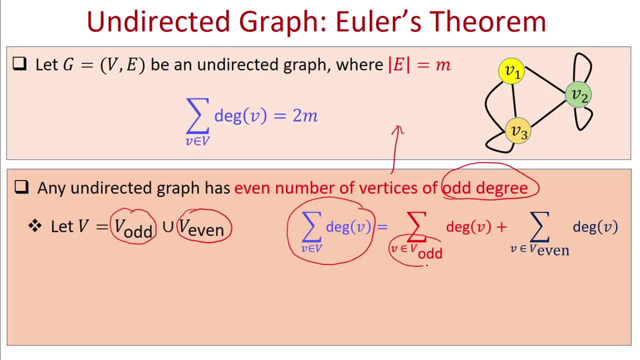 You take all the vertices in the set V-odd, namely all the vertices which have odd degrees, and take the summation of the degrees of the respective vertices in the set V-odd. And you take all the vertices in the set V-even, namely all the vertices which have 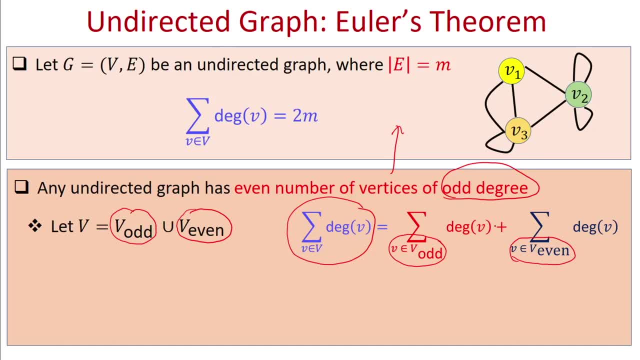 even degrees and sum of their degrees, And if you sum these two quantities, that will give you the summation of the degrees of all the vertices in the graph. Now I know that the left hand side of this equality is even because, as per the above theorem, 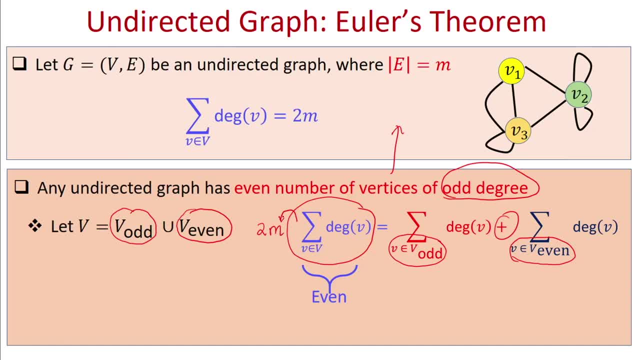 the left hand side is two times the number of edges. The number of edges could be odd, it could be even. But two times that number of edges will be an even quantity. So I know that the left hand side is an even quantity. 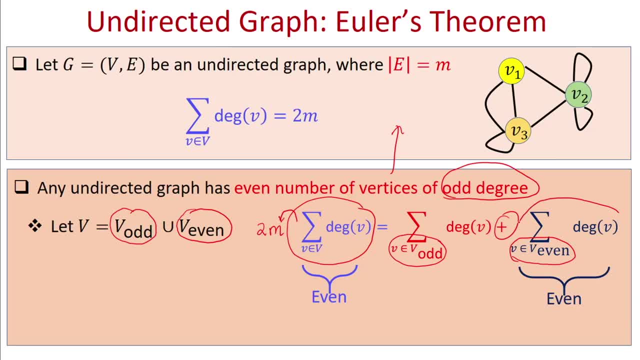 And I also know that if I sum up the degrees of all the vertices which have even degrees, then that is also an even quantity, The number of vertices of even degree. it could be odd, it could be even, it doesn't matter. 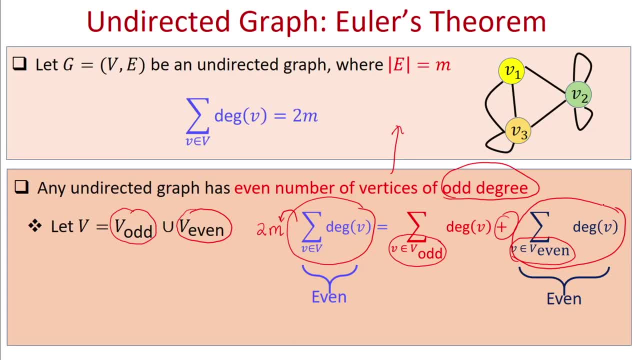 But since I am adding even number of, but since I am adding several quantities, each of which is an even quantity, the overall summation will be even. From that, I can conclude the following: that I can conclude that, if I sum up, 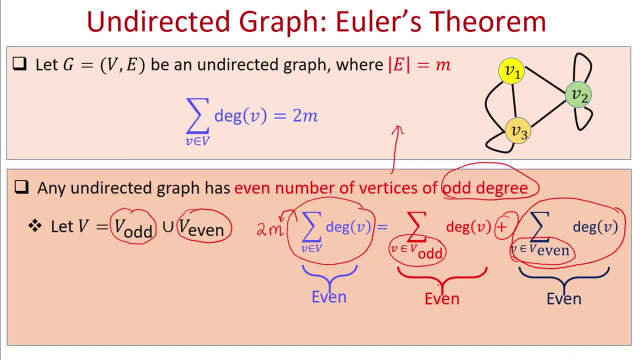 the degrees of all the vertices in the set V-odd, that also will be even, because if that is not the case, then you can't have the difference of two even quantities, because that is simply coming from the fact that the summation of the degrees 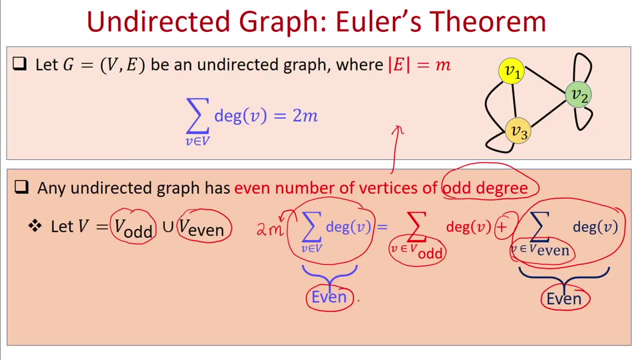 of all the vertices in the set. V-odd is the difference of two even quantities, And the difference of two even quantities will be even. So what is the conclusion that we have drawn till now? We have concluded that, if I take the summation of degrees of all the vertices, 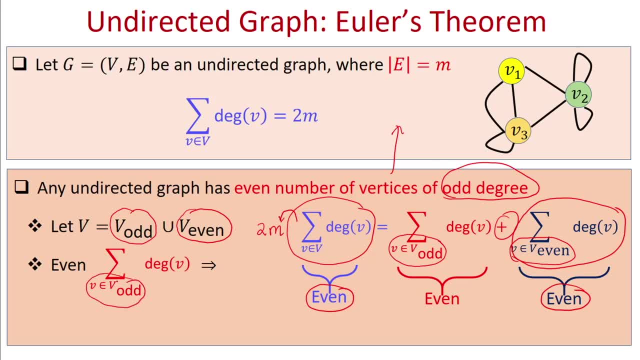 in the set V-odd, then that is an even quantity And that is possible only when the number of entities in the set V-odd is even Right. So, because you are summing up several odd quantities and the summation of those odd, 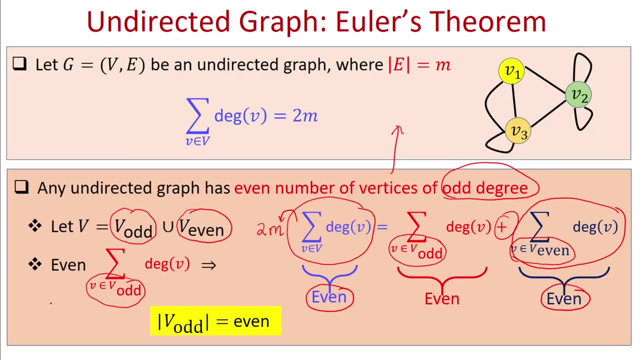 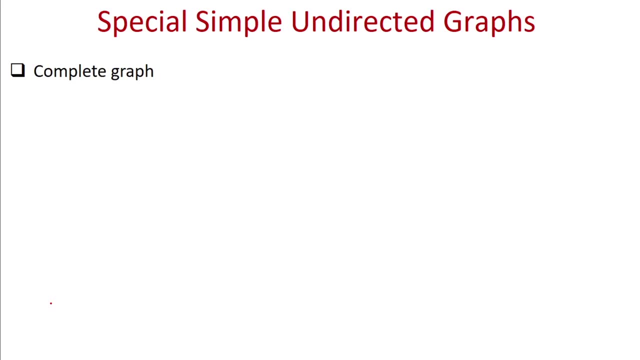 quantities is even. that is given to you. that is possible only when the number of quantities that you have added is even. So that's a fundamental fact about any undirected graph, irrespective of whether it is a simple graph or a non-simple, or whether it's a regular. it's not a simple graph. 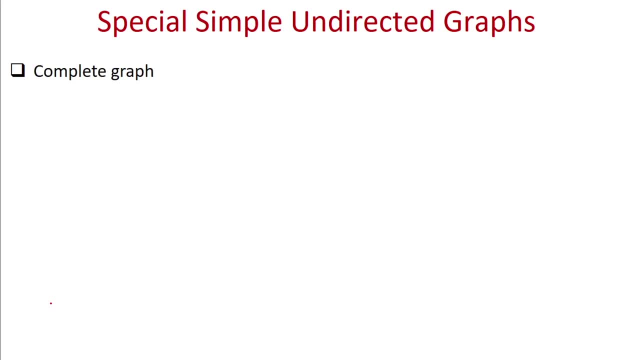 OK, Now let us define some special types of undirected graphs. So the first special type of undirected graph is a complete graph, And the property of this graph is that you have exactly one edge between each pair of distinct vertices. And since this is a simple graph, OK. 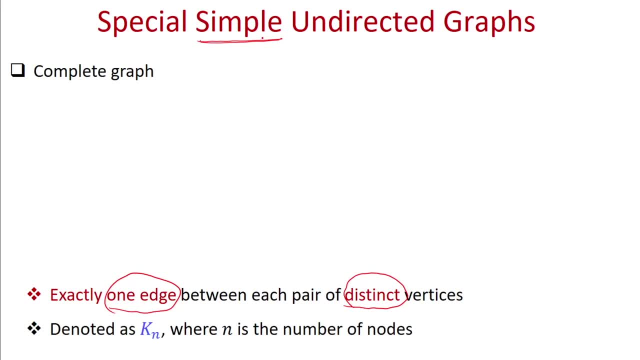 and our property is that you can't have more than one edge between every pair of distinct vertices. automatically we have here the restriction that you can't have a self-loop, because if you have a self-loop, then that self-loop will be violating the definition here. 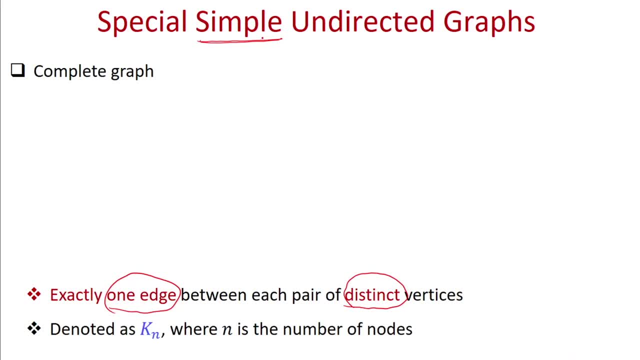 So the requirement here is that you take the vertices, all the vertices, between every pair of distinct vertices. you will have exactly one edge. You don't have the option of zero or one edge. Exactly one edge should be there between every pair of distinct vertices. 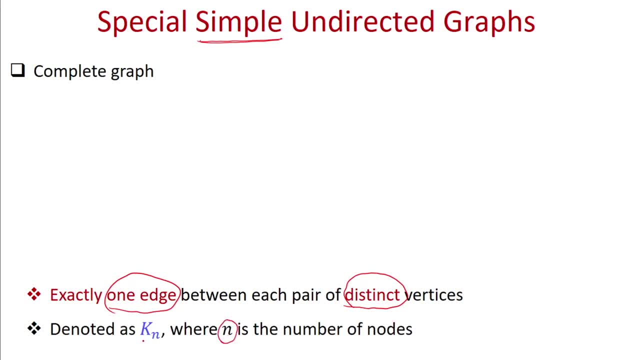 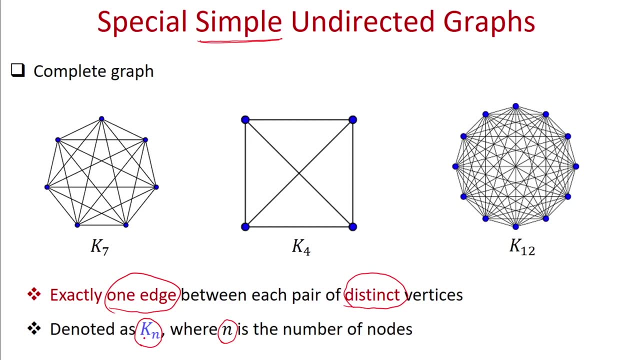 And if n is the number of nodes in a complete graph, then we use this notation k sub n to denote a complete graph with n nodes. So these are the examples, some of the examples of complete graphs with various values of n. the complete graph with 7 nodes is this: 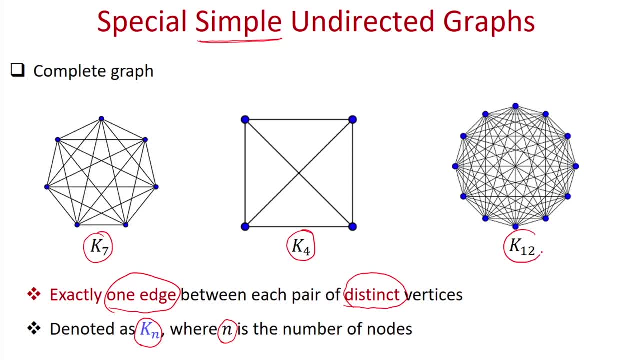 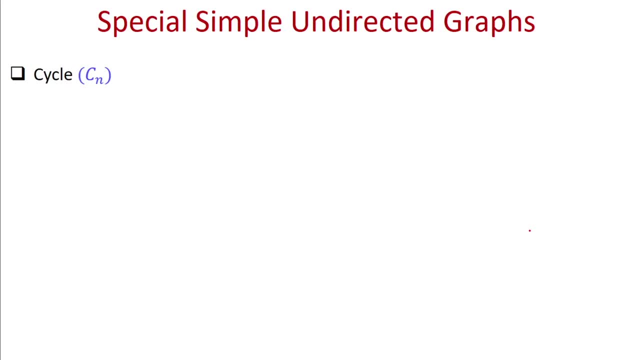 complete graph with 4 nodes? is this complete graph with 12 nodes? is this, Then, another special type of simple, undirected graph is a cycle graph, denoted as cn. Here, the vertex set will be consisting of n nodes and you will have edge set of the form. 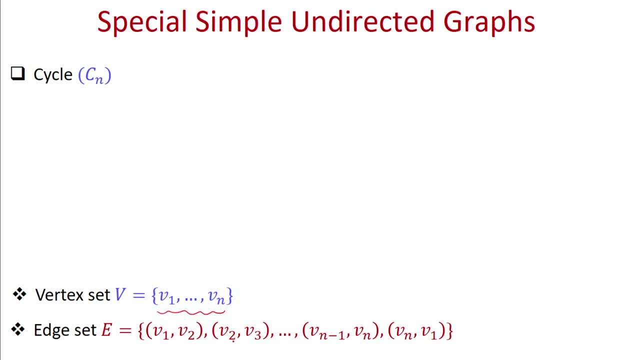 of the following: you will have an edge between the vertex 1 and 2.. You will have an edge between 2 and 3.. You will have an edge between the n-1th vertex and vertex vn, And then you will have an edge between the vertex vn and v1.. 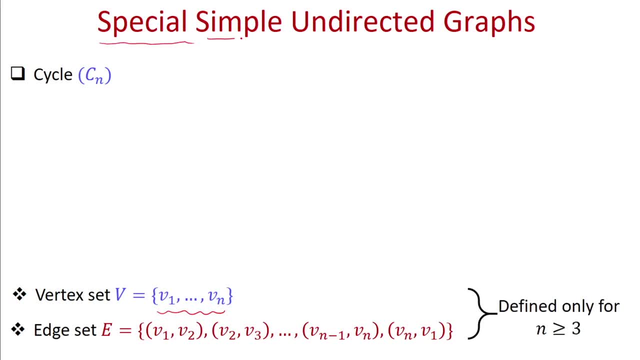 Now, since the graph is simple, ok, the cycle graph is defined only when the number of vertices is n is greater than or equal to 3, because if I try to define a cycle graph involving just two nodes, then, as per the definition, the edge set will be the following: 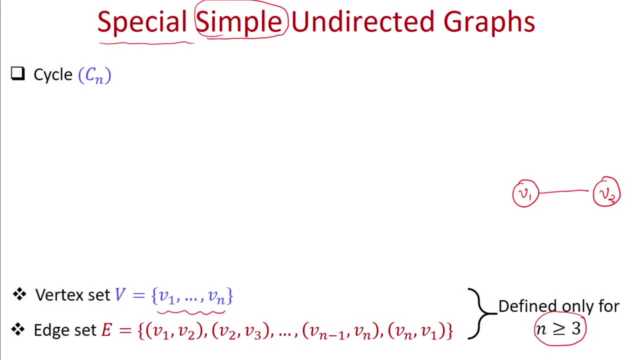 You have an edge between 1 and 2.. And again you have an edge between 2 to 1.. OK, that will be the definition of the edge set as per this general definition, But that will violate the property that it is a simple graph. 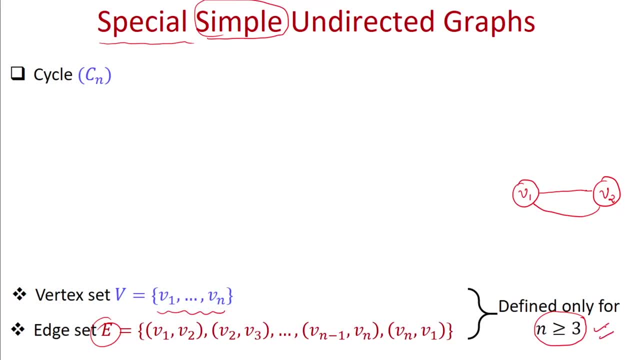 So that's why n is greater than or equal to 3.. And then only we can define a cycle graph. Well, you can't say that. why can't I take this to be a cycle graph, namely a graph where I have just an edge between 1 and 2, because the interpretation of the cycle 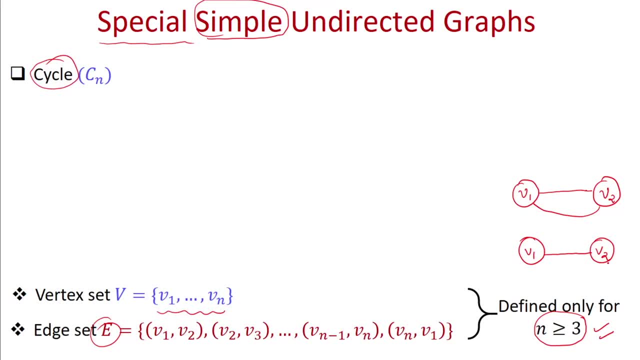 here is the following: the interpretation of the cycle is that once you go to the n-th vertex, you have an edge from the n-th vertex back to the first vertex. OK, so, without violating the requirement that your graph is a simple graph, 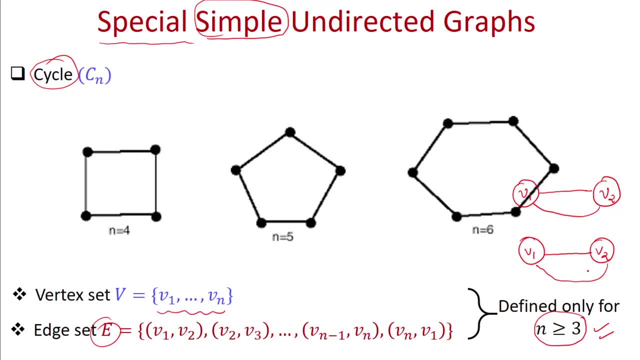 this is possible only when n is greater than or equal to 3.. So if I consider a cycle graph with three nodes, then that will be something like this: You have v1, v2, v2, v3, and then you have an edge back from 3 to 1.. 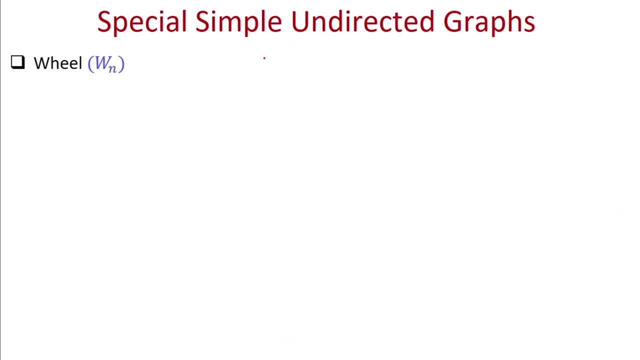 Then there is another special, simple, undirected graph called as the wheel graph, So it is slightly different from the cycle graph. So what you do is you take a cycle graph involving n-th nodes and then you add a central vertex, which is the n-th vertex, and the central vertex is now. 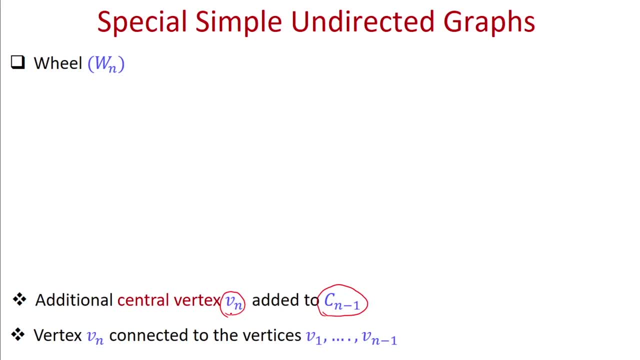 we add an edge involving the central vertex and all the vertices in your cycle graph c of n-th. So, for instance, if I want to form w4, then I take the cycle graph involving three nodes, add the fourth vertex, v4, and add an edge from this fourth vertex. 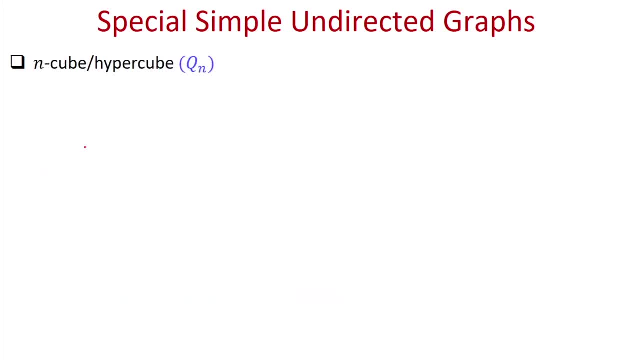 to every other existing vertex in the cycle graph. We also have another special, simple, undirected graph called as the n-cube or the hypercube, denoted by this. So this is the representation q of n. So this graph will have 2 to the power n nodes, where each node represents: 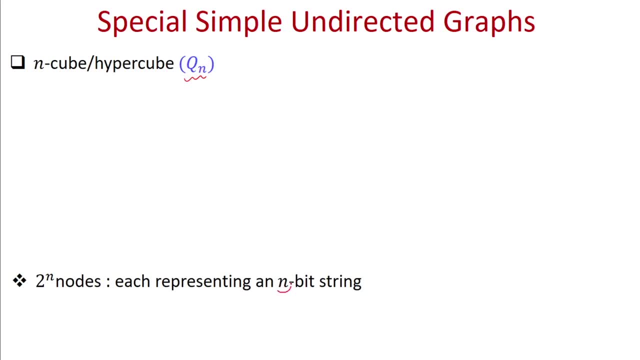 a possible n-bit string. So remember that the number of bit strings of length n is 2 to the power n. So each string is represented by a node in this hypercube graph And you have an edge between the i-th vertex and the j-th vertex. 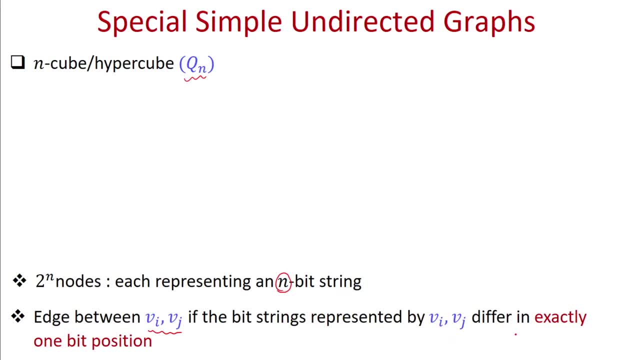 So you can see that if the bit strings represented by the i-th vertex and the j-th vertex differ in exactly one bit position, otherwise the edge is not there between the i-th vertex and the j-th vertex. So, for instance, if I take the graph q1, then I can have only two strings. 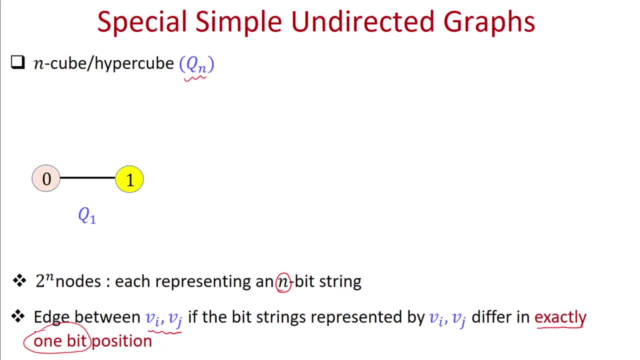 two bit strings of length 1,- the bit string 0 and the bit string 1, and they differ in exactly one bit position, so the edge will be there. If I want to form the graph q2, the way I do it is as follows. 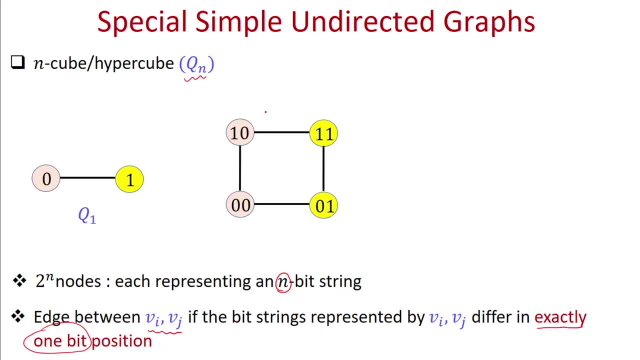 So there will be- this will be the graph q2.. Okay, because you will have four strings of length, four bit strings of length 2.. And you can see that this edge is there because the binary string 1: 0 differs with the string 0: 0 in exactly one bit position, namely the first bit position. 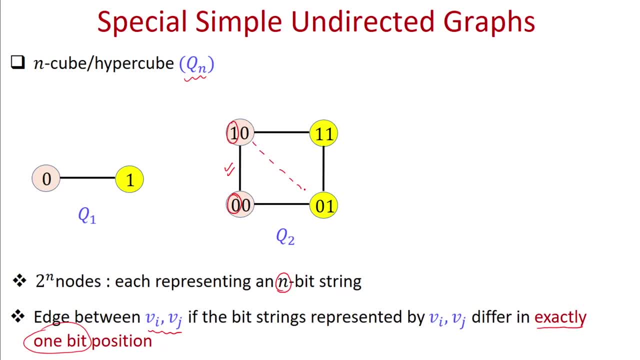 You don't have an edge between the bit string or the vertex representing the bit string 1- 0 and the vertex representing the bit string 0- 1, because these two bit strings differ in more than one position. So let me go back and try to understand. 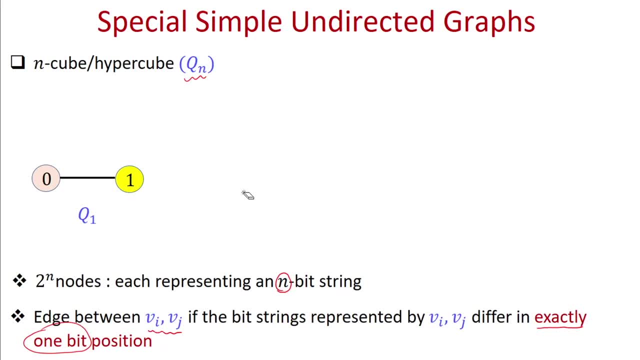 that, what exactly is the relationship between q2 and q1, how exactly I can interpret q2 or relate q2 with the graph q1.. So the way I can construct the graph q2 is as follows. I take two copies of the graph. 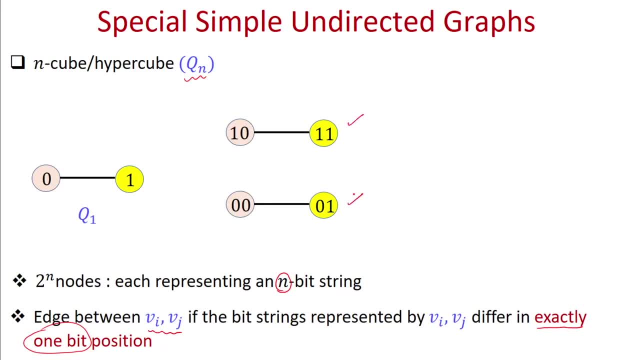 q1.. This is your first copy and this is the second copy. In the first copy I add the bit 1 at the beginning of all the nodes, or all the bit strings represented by the nodes in the copy of q1, right. 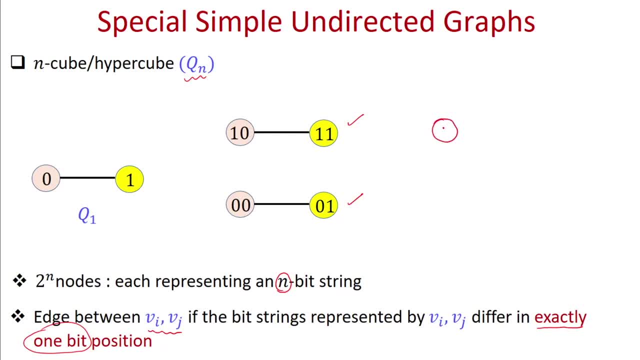 So the copy of q1 that I would have taken is the following: I would have taken the vertex representing the bit string 0, the vertex representing the vertex bit string 1.. What I'm saying is you add a 1 at the beginning of these bit strings. 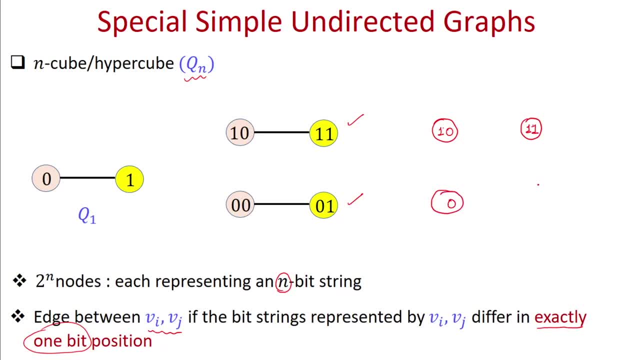 You take the second copy of q1 and you add a 0 at the beginning of all the strings represented by the nodes in this copy of q1.. And now you add the required edges depending upon the bit strings. So you can see that the edges differ in exactly one bit position or not. 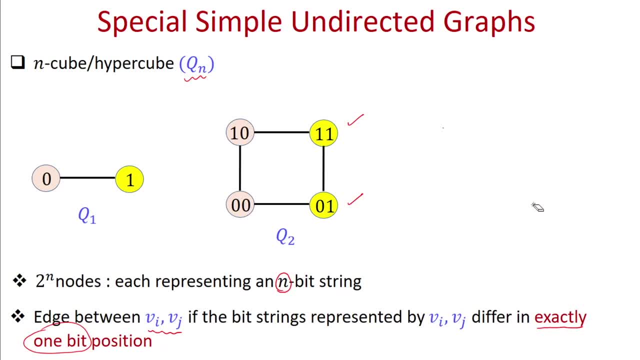 OK, In the same way, if I want to get to, if I want to define or get the graph q3, what I do? the following: I take two copies of q2, one copy of q2, another copy of q2 and I extend the length of the bit strings of the nodes. 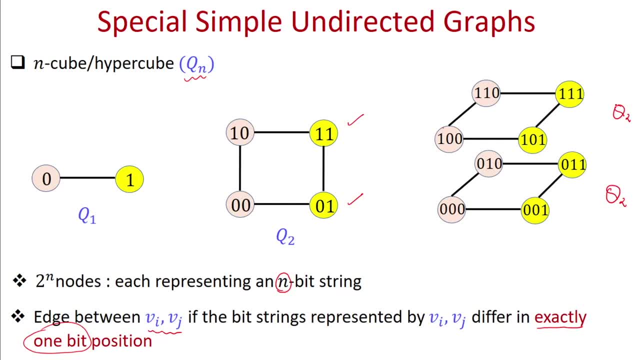 by adding 1 at the beginning of all the strings in the first copy of q2.. And I add 0 at the beginning of all the bit strings in the second copy of the q2 and then I add the required edges, depending upon whether the two vertices 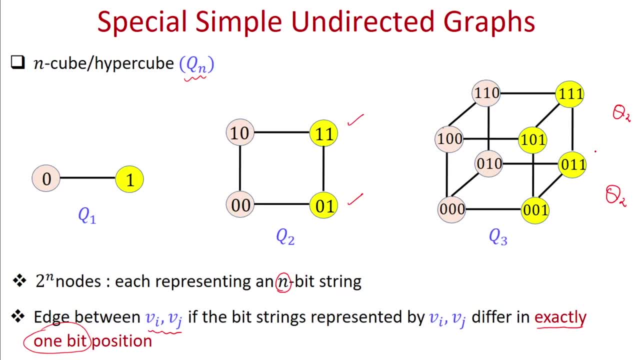 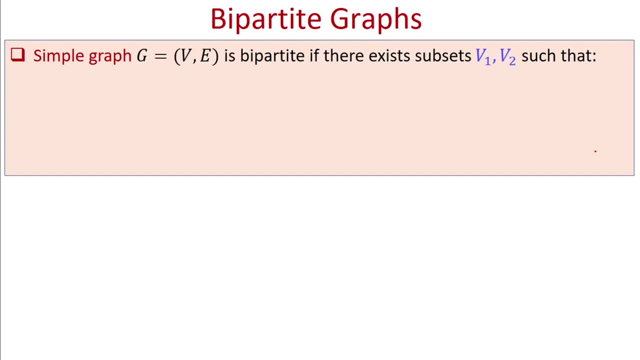 differ in exactly one bit position. Right, That's the definition of our q1 graph. Now let us define what we call as bipartite graphs. So if you are given a simple graph, OK, Then the graph is called bipartite. if 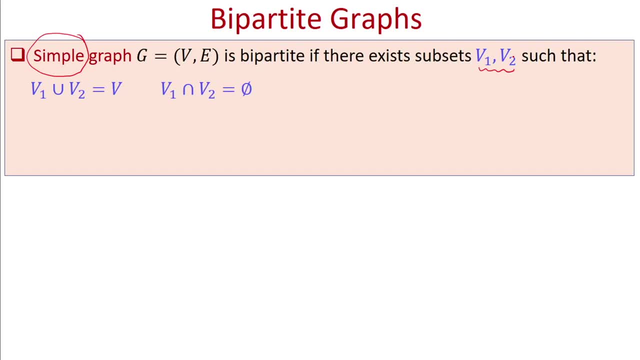 we can find out two vertex sets, v1 and v2, such that the following would: The vertex sets v1 and v2 should constitute a partition of your vertex set. That means the union of v1 and v2 should give you back the original vertex set. 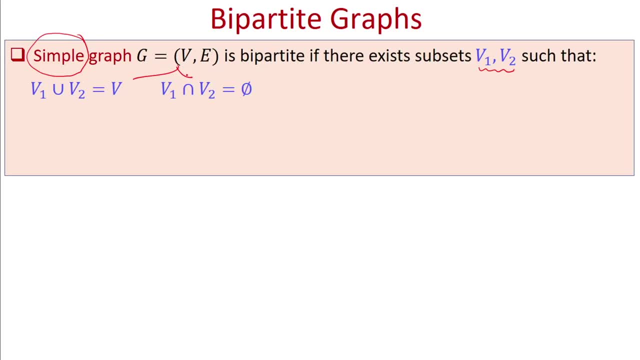 And there should not be any overlap or intersection between the vertex sets v1 and v2.. And the second property that I need from this partition v1, v2 is the following: I need the following: You take any edge e in the graph with endpoints whose endpoints are vi and vj. 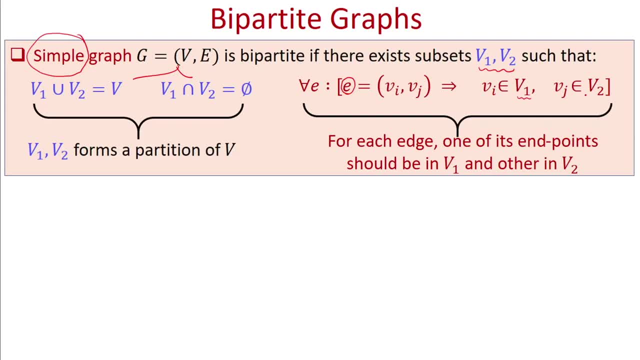 then one of the endpoints should be in one of the subsets and the other endpoints should be in the other subset. So what it means is that you take any edge of the graph. It can't be the case that both its endpoints are in the same set, v1 or v2.. 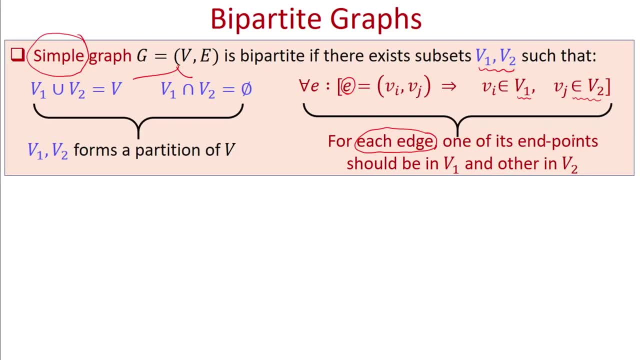 One of the endpoints should be in v1.. The other endpoints should be in v2.. OK, so, for instance, if I take this graph, then this graph is not a bipartition graph. It's not a bipartite graph because I can't find the required v1 set and v2 set. 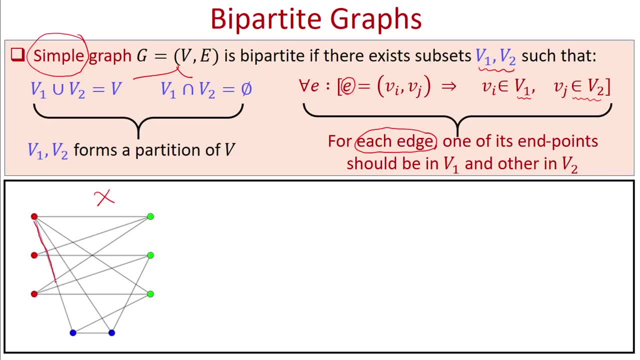 This is because, if I focus on this specific portion of the graph, namely this portion is the triangle graph. OK, so if I call these edges as e1, e2 and e3, and if I try to find out a candidate- v1, v2- satisfying this condition, 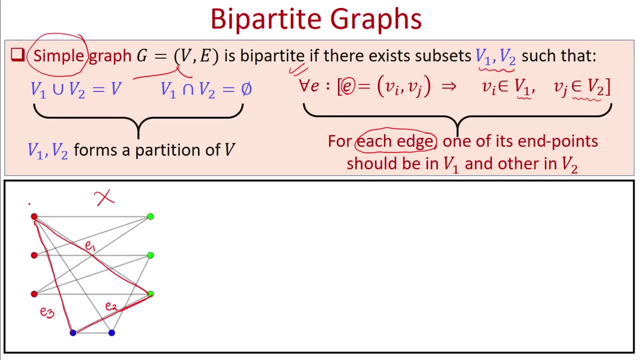 I can't do that. Say, for instance, I include this red colored vertex in the set v1.. So let me call these vertices as a, b, c. So suppose I include a in v1, as per my requirement, since the other end point of edge e1,. 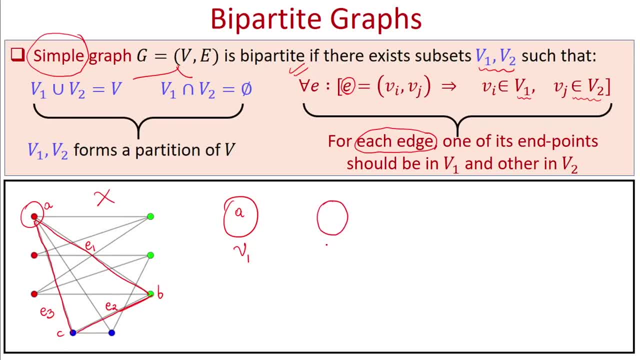 the vertex b should be the other subset or other partition. I should put the vertex b in the subset v2.. That's fine. Now what about the edge e2? The other end point of the edge e2 is c, So it can't go in the same set v2 because that will violate my requirement. 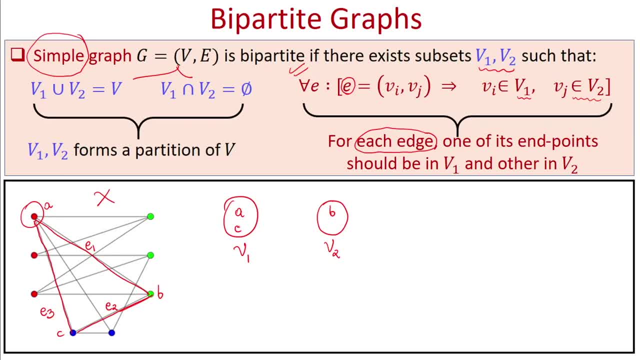 So I can put c in the collection v1.. But as soon as I put c in the collection v1, I see that I get a violation, because I now have an edge, namely e3, where both the end points a and c are in the same collection v1. 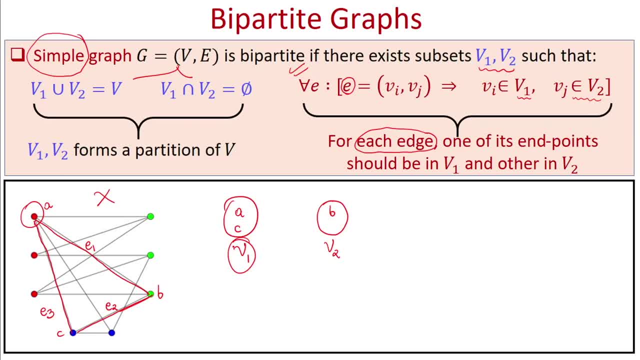 Right. So that's why, irrespective of how you try to come up with your candidate v1 and v2, you can't find a partition v1, v2 for this graph satisfying this requirement. So that's why this graph is not a bipartite graph. 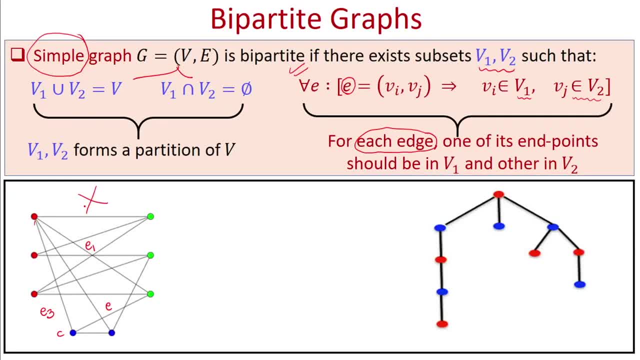 But if I take this graph, then this graph is a bipartite graph And what will be the partition set for the vertex set v? What you can do is you take all the blue colored vertices and put them in the collection v1.. 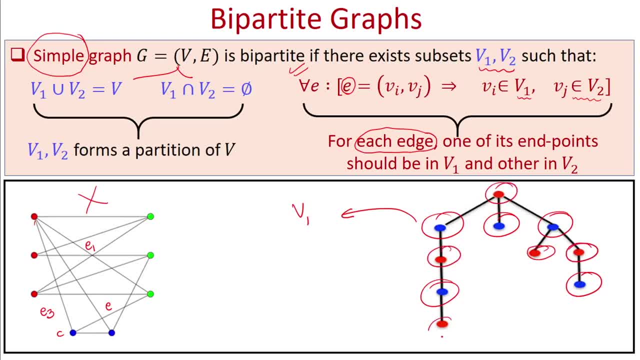 And you take all the red colored vertices and put them in the collection v2.. And now you can see that you take any edge e in this graph. one of its end point will be in this v1. And the other end point will be in v2.. 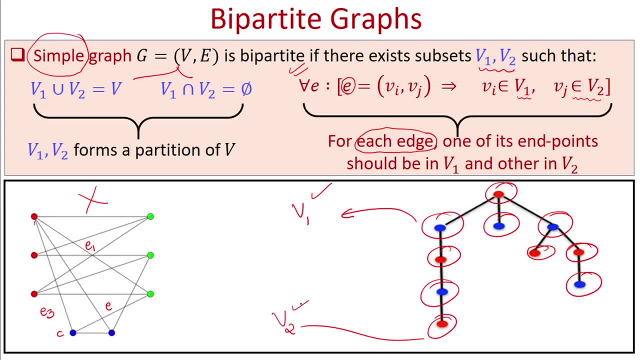 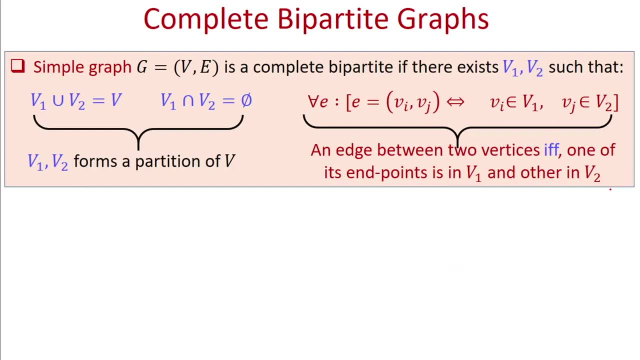 It won't be the case that both its end points are either in v1 or in v2.. So that's why this is an example of a bipartite graph. Now let's define next what we call as a complete bipartite graph. 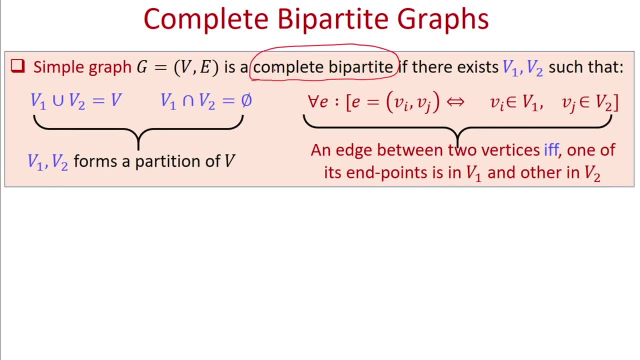 So it is a special type of bipartite graph. So, first of all, it is a bipartite graph. Namely, it should be possible to come up with a partition of the vertex set, And that partition should have a special property. 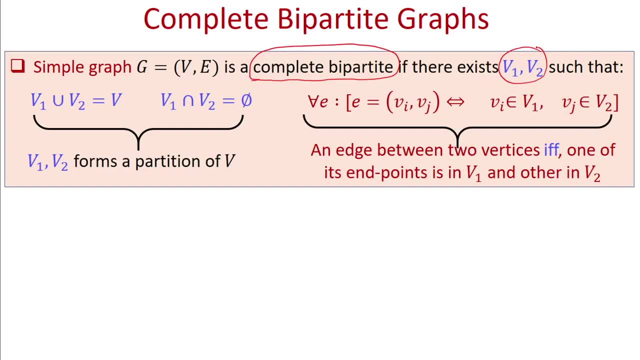 Now you take any edge in the graph, One of its end point should be in v1, other end point should be in v2.. That comes from the definition of the bipartite graph. But this implication is now a bi-implication. 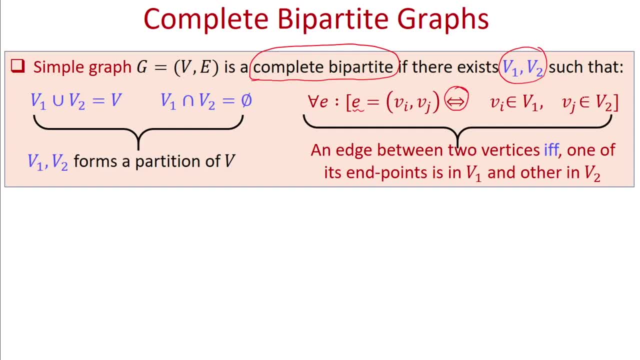 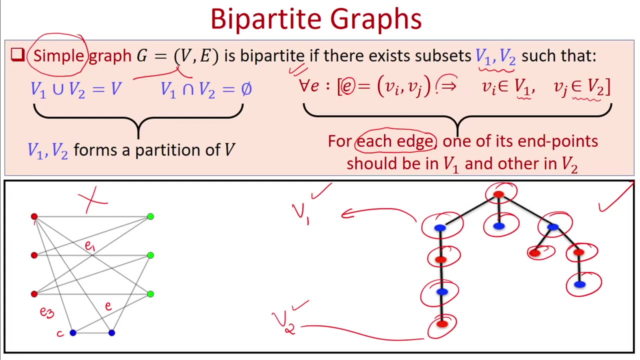 That means it is the case that you have an edge in the graph between each and every vertex in the set v1 and the set v2.. So if you compare this bi-implication condition with the previous definition in the previous definition it might be possible that you have some. 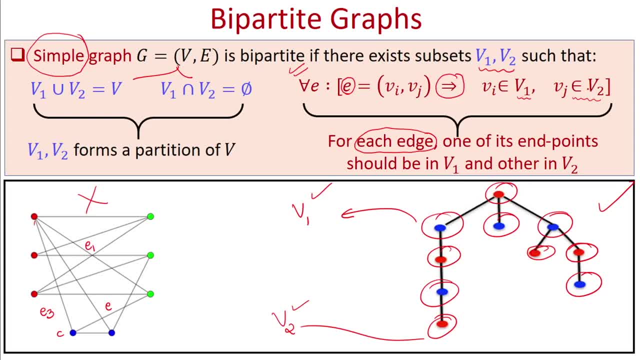 vertices in v1 and some vertices in v2, such that between those vertices you don't have an edge in the graph. So, for instance, if I take this graph, then this is a bipartite graph, but this is not a complete bipartite graph. 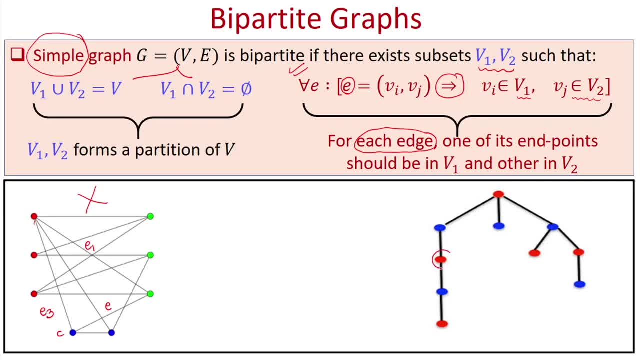 Why it is not a complete bipartite graph? Because you say, for instance, you take this vertex, it will be in one of the subsets given by your partition and you take this blue colored node, This will be in the other subset in your partition, but you don't have an edge. 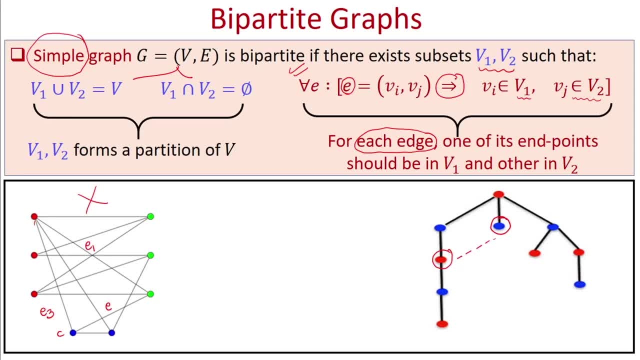 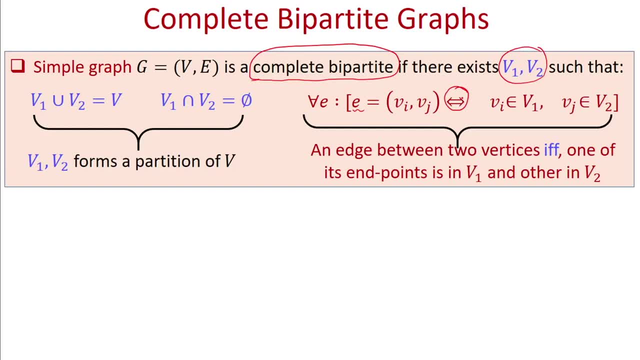 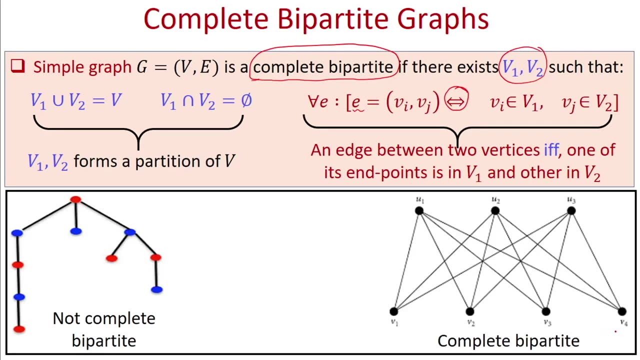 between these two vertices in the graph. So that's why this implication was there only in one direction. But in a complete bipartite graph, what I'm saying is the implication should be a bi-implication. OK, so that's why this graph is not a bipartite graph, but this graph is a.